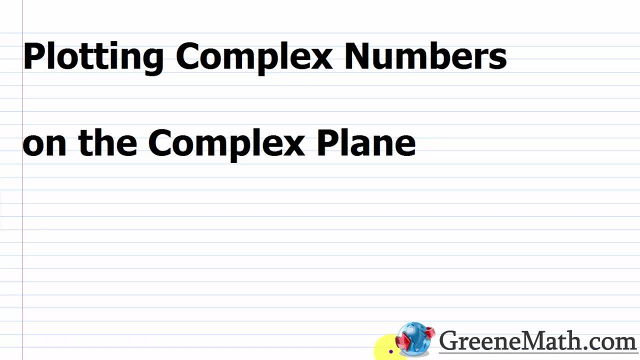 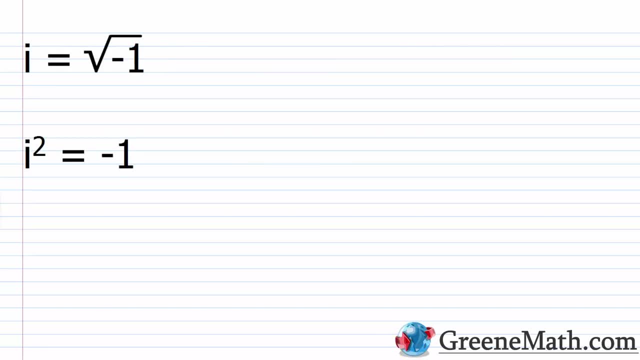 In this lesson we want to talk about plotting complex numbers on the complex plane. So at this point in our course we already know and understand how to use the imaginary unit i. i again is defined as the square root of negative 1, or you could say i squared is equal to negative. 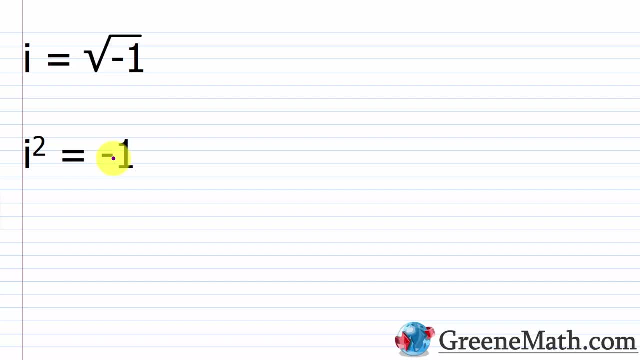 1. So we found that this came in handy when we're solving quadratic equations, right? In some situations, you won't be able to get a real solution, and so you need to turn to the imaginary unit i to gain a solution. Now we have also talked about complex numbers and complex numbers. 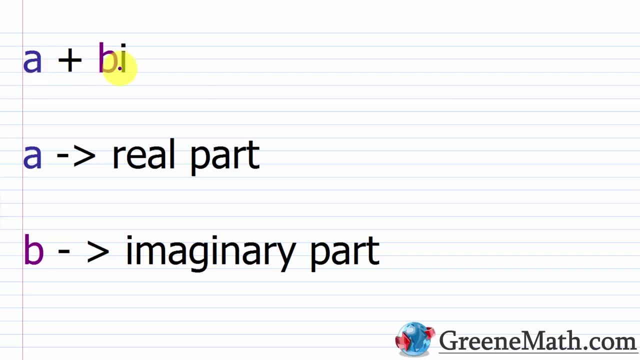 are of the form a plus bi. So we've seen these before, we've performed operations with them before, and we should know that a- this part right here- is known as the real part of the complex number and b- this part right here that's multiplying i, the imaginary unit, is known as 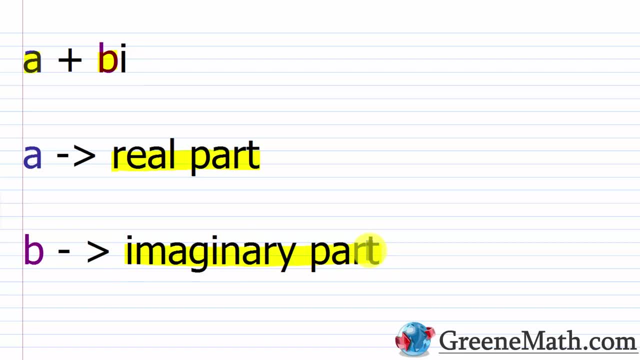 the imaginary part of the complex number. Now some books will say bi is the imaginary part. but for the purposes of this lesson we're going to talk about the imaginary part of the complex number. We're just going to stick to saying that b is the imaginary part. Now how can we plot a? 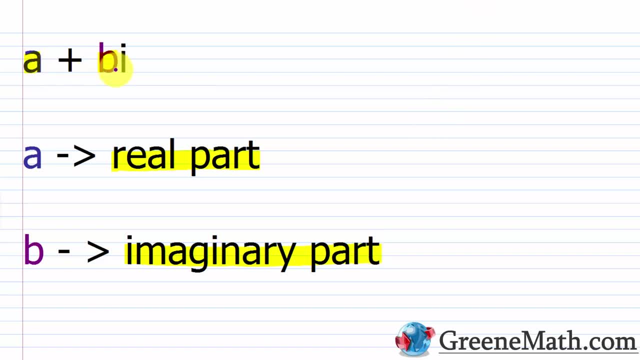 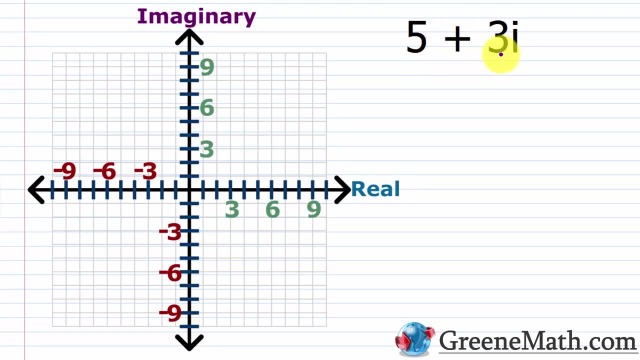 complex number, such as a plus bi on the complex plane. Well, let's go down to our complex plane and suppose we wanted to plot something like 5 plus 3i. Well, I'm just going to kind of match this up real quick. I'm going to say: this is a plus bi, so my a here is 5, and my b here is 3,. 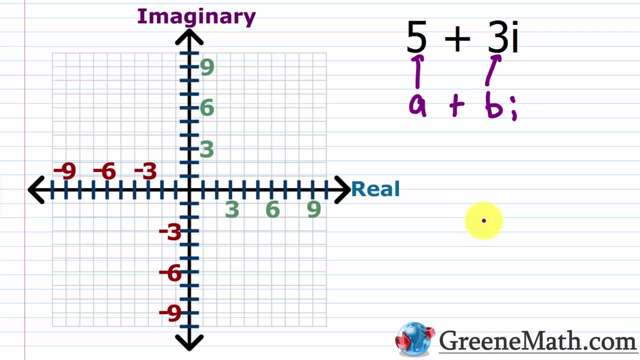 okay, So keep that in mind. Now the complex plane. looking at it, you might say: well, that looks just like the coordinate plane I'm used to working with. when we see real numbers, Well it does. It looks exactly the same. The difference is: 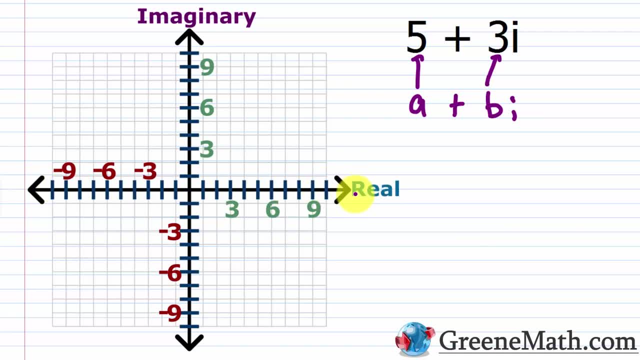 is that instead of the horizontal axis being labeled with x, now it says real. Instead of the vertical axis being labeled with y, now it says imaginary. So it's very easy to plot 5 plus 3i: Again the a or the real part is 5.. So on the real axis I'm just looking for 5.. So that's. 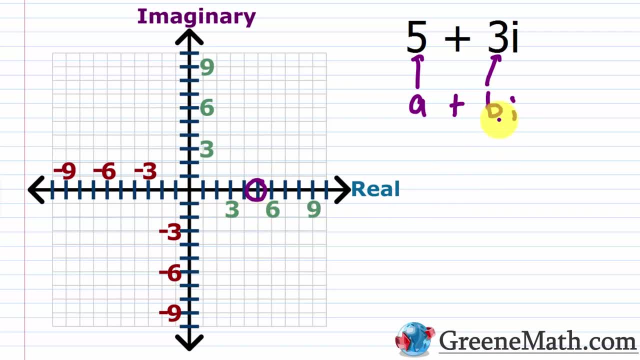 going to be right here. So I'm just going to circle that. Then I'm looking for 3 on the imaginary axis, because the b here, or the imaginary part, is 3.. So on the imaginary axis I'm just going up 3, so that's right here And I'm just finding. 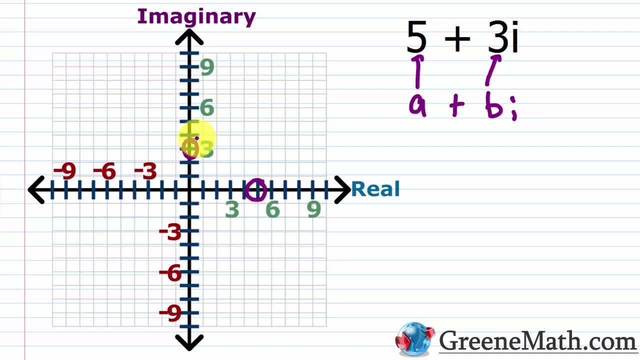 the meeting point between the two. So this is just like if I had 5 comma 3 in the real number system. It's the same process, okay, So I'm going to go 5 units to the right on the real axis. 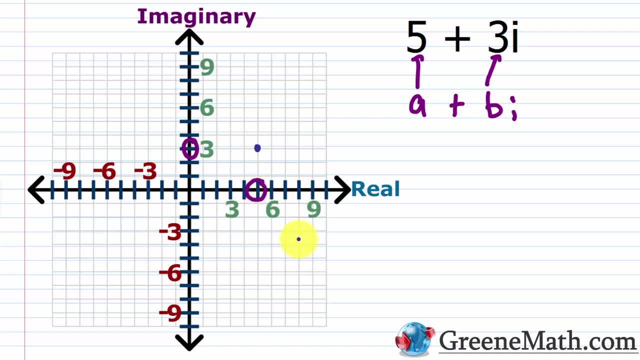 and 3 units up on the imaginary axis. So I'm going to be right here. This is going to be my 5 plus 3i. okay, It's just that simple. All right, let's go ahead and try another one. 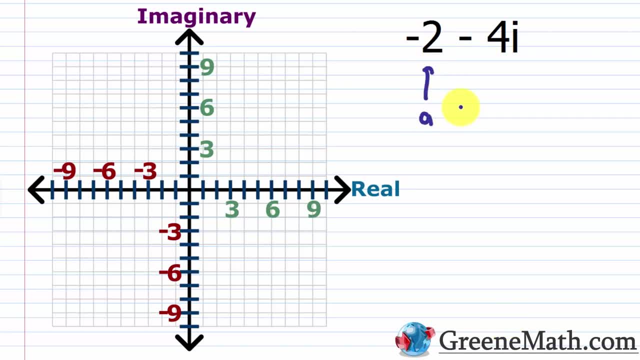 So again, I'm going to write this in the format I'm going to say: this is a plus bi. okay, Now, in this case my a is negative 2.. So that means on the real axis I want to go 2 units to the left. 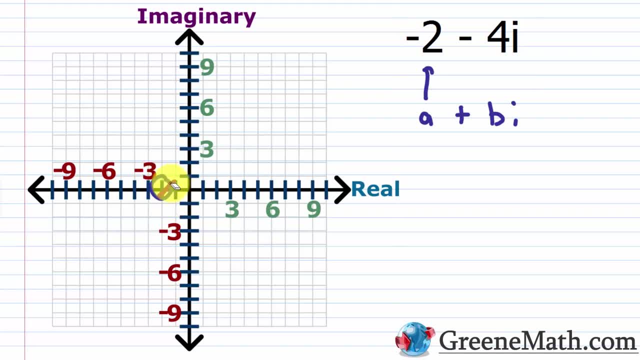 So that's going to be right here, And let me use a different color, because that doesn't show up very well. So let me use kind of a reddish or purple. I'm not sure what you'd call that color, Maybe it's magenta, And then for my b, I'm thinking about the fact that this is negative. 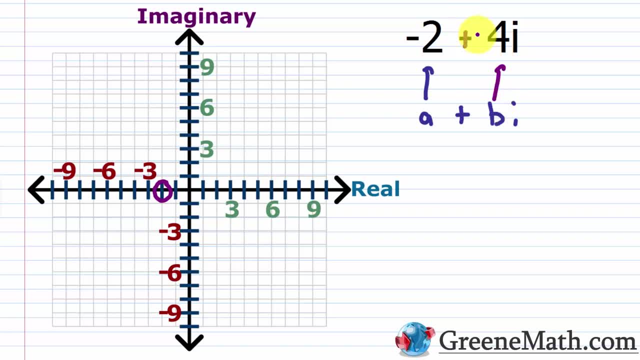 So really, if I want to stay consistent with this, I'm going to write this as plus negative 4i. okay, So my b here is a negative 4.. So that means I want to start on the imaginary axis at 0, and I want to drop down 4 units. So that's going to be right there. So this is just. 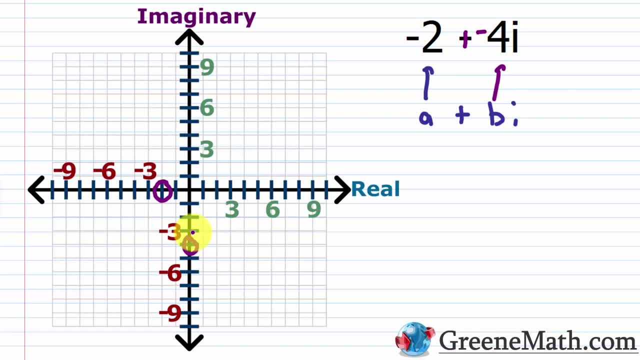 like if you had negative 2 comma, negative 4, if you were working in the real number system. So I'm just going to go 2 units to the left on the real axis and I'm going to go 4 units down on the imaginary axis and that's going to be right there. So this is going to be my negative 2,. 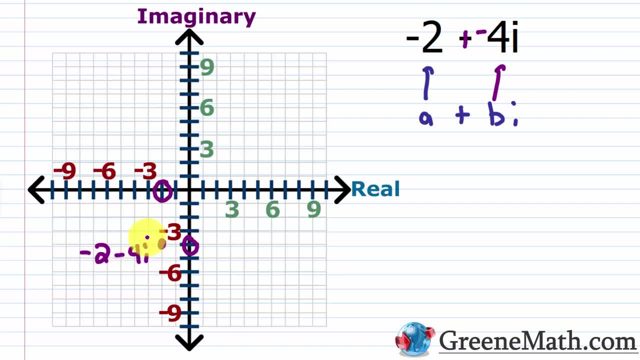 and then I'll put minus 4i. Again, you could put plus negative 4i. It doesn't. it doesn't match the same thing. All right, what about 8 minus 6i? So again, let's just match this. 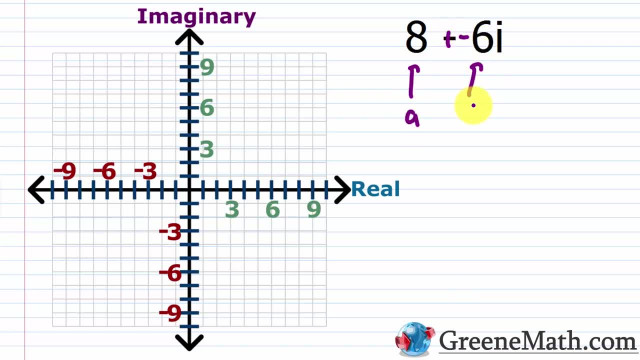 up. This is my a, and again I'm going to put plus negative here. This is my b. okay, So I want a real location of 8.. So I'm going to go 8 units to the right on my real axis. So that's here. 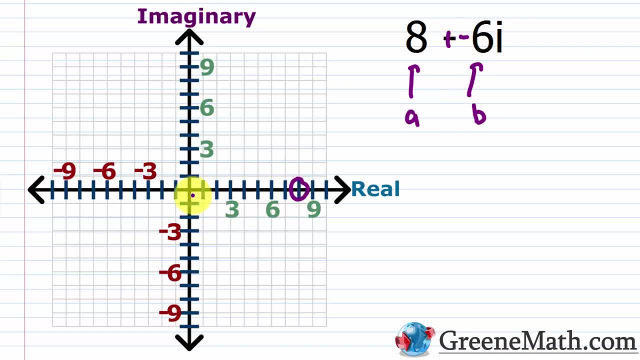 And then I want a negative 6 for my imaginary axis. So I'm just going to go down 6 units, So that's going to be right there. So I go 8 units to the right on the real axis and 6 units down on the imaginary axis. So that's right there, And this is going to be 8. 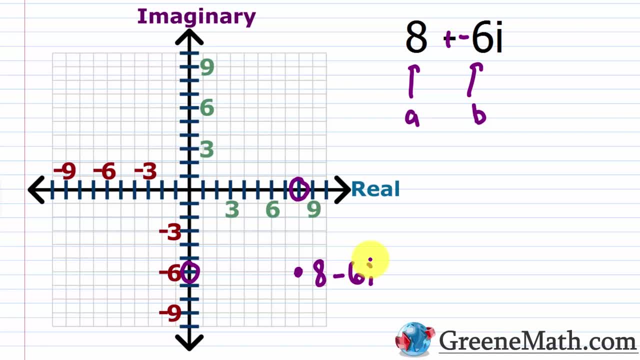 minus 6i, 6i, or again 8 plus negative 6i. All right, so let's look at another one. So we have negative 5 minus 7i. So this guy right here is my a, and again I'm going to put plus negative here. So 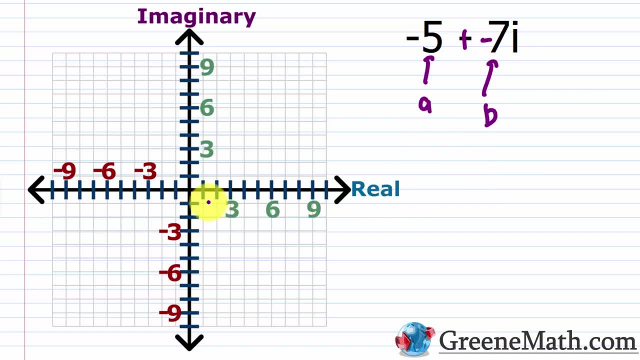 that's going to be my b. So again, on the real axis, I'm going to negative 5.. So that's going to be right here. On my imaginary axis, I'm going to negative 7.. So I'm going to drop 7 units. 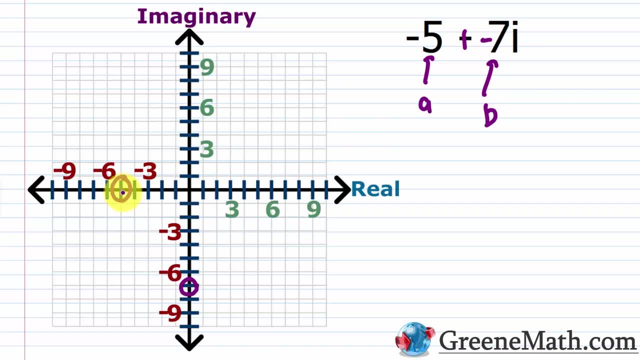 That's here. So again, 5 units to the left on the real axis, 7 units down on the imaginary axis. That's going to be right there, And let me label this below it. So I'm going to put negative 5, and I'm going to do minus 7i. So that's that point, right there. 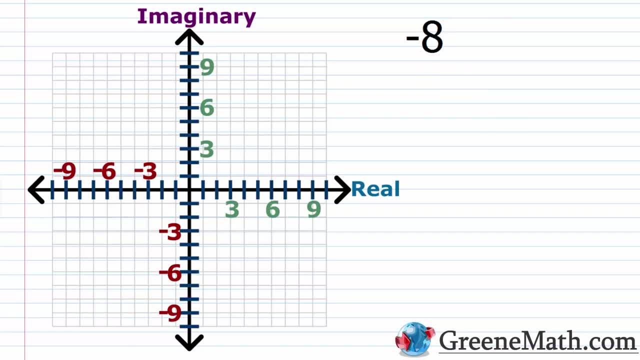 Okay, so what if they throw a curveball at you? This is one that kind of trips people up a lot. Let's say you're working on a complex plane and someone says, to plot, negative 8.. What do you do? Well, some of you will immediately say, okay, well, I know that. 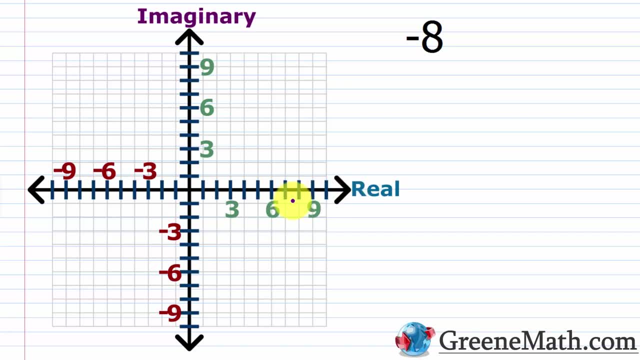 negative 8 is a real number. So I'm probably just going to go to negative 8 on the real axis and I'm just going to put a point there And you'd be correct. But another way you can think about is you can still follow the format of a plus bi. okay, Because a here is negative 8,. 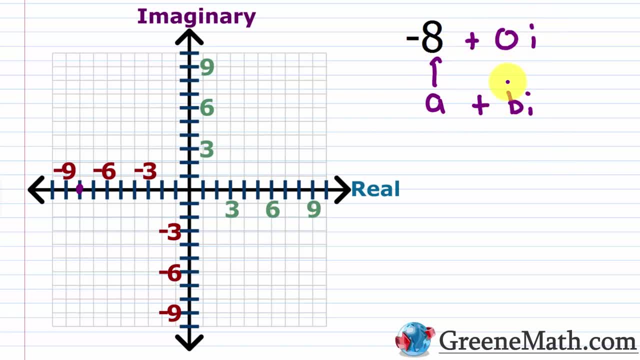 but I can say plus 0i, okay, And so my b here is just 0.. So if I go 8 units to the left on the real axis and 0 units up on the imaginary axis, I am at this negative 8 on the real axis, okay. 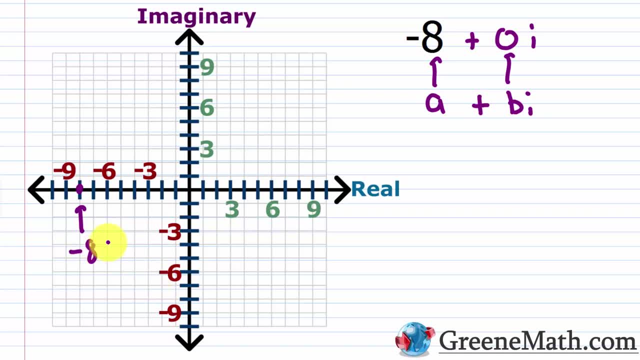 So this right here would just be negative 8, or you put negative 8 plus 0i if you wanted to write it in the complex number form. What about something Just like 9i? Well, again, we can use the same technique. We can write this as a plus bi by just. 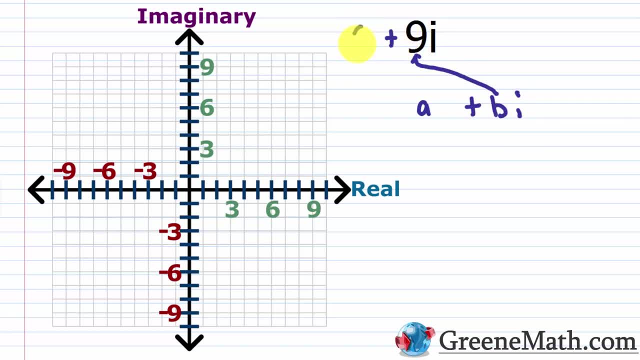 saying that this is my b here, So I can put a plus here and I can just put a 0 here. okay, So my a here is just 0.. So that means on the real axis I'm not going to move at all, I'm not going. 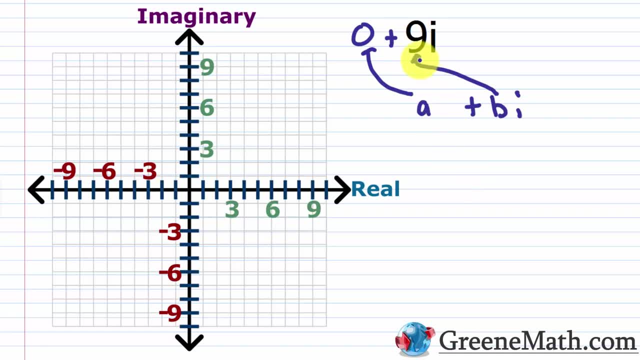 left or right at all. okay, All I'm going to do is I'm going to travel 9 units up on my imaginary axis, So I'm just going to go up 9 units, So I'm just going to place my circle there and this will. be 0 plus 9i.